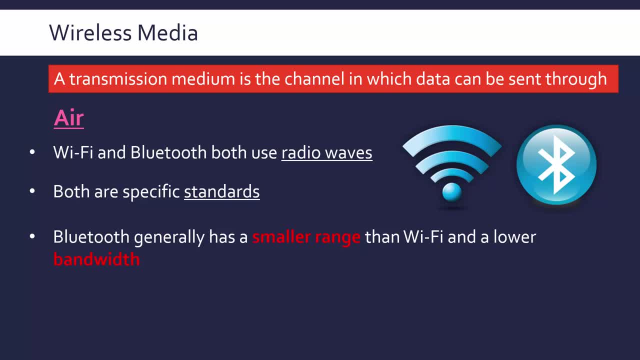 using Bluetooth. There is nothing special about Bluetooth itself. Bluetooth is just a standard which has become quite popular. You could use other frequencies, it's just. Bluetooth is quite widely supported. Now, another downside to Bluetooth is it has got a lower bandwidth, generally speaking, than Wi-Fi. 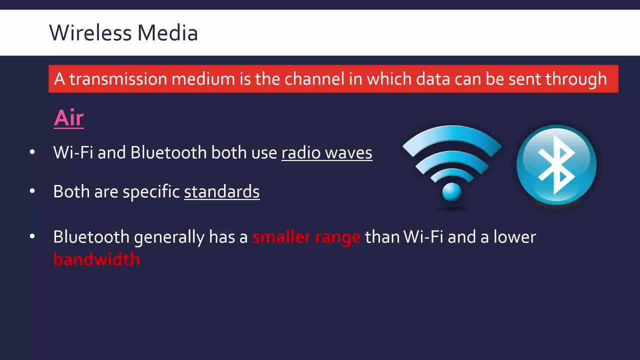 The bandwidth is all about how much data you can fit through the network at any given point. but if we were to evaluate Bluetooth versus Wi-Fi, actually Bluetooth is what we could describe as ad-hoc. An ad-hoc network is a network which you can set up very quickly and very easily. Setting up a Wi-Fi network, 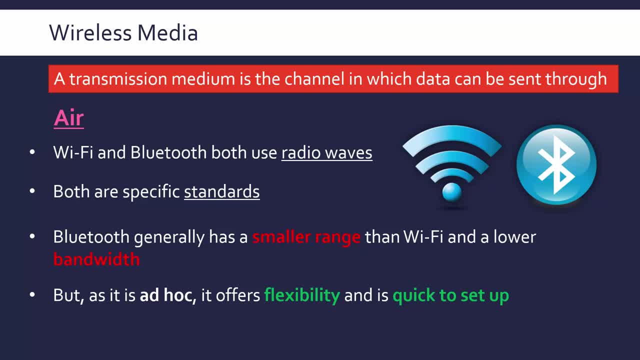 is not exactly rocket science but, as you might know from experience, can take some time. You've got to install a wireless network adapter. you've got to plug in the wireless router to a particular area of your home where you've got a port. It's not as flexible as 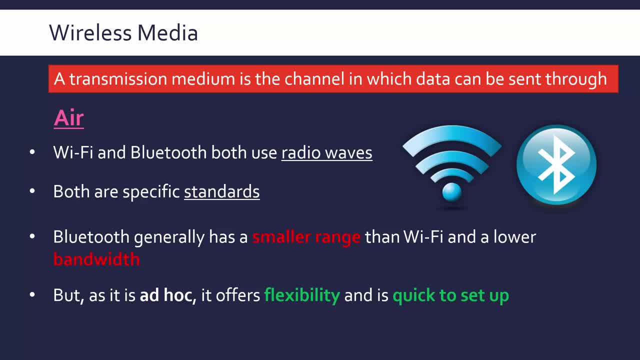 compared to Bluetooth, which you can just toggle on and off on your phone, say, Very easy and flexible to set up, so that is definitely an advantage of Bluetooth. Now, that is a quick comparison between Bluetooth and Wi-Fi, but generally you can compare wireless to wired. That's quite a common exam. 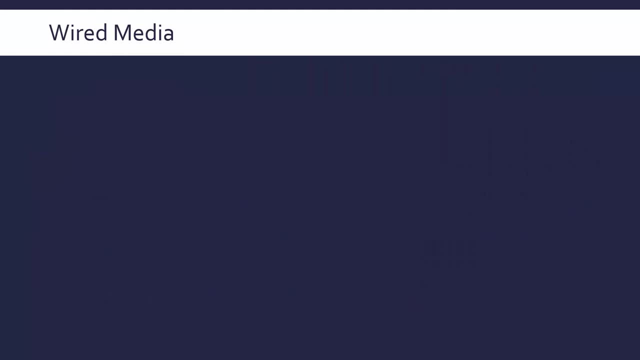 question to consider: is it more suitable to go for a wired network or a wireless one? I will leave that evaluation for another video, because right now I just want to go over two common examples of wired media, The first of which are copper cables. A cable is just a series of parallel wires. 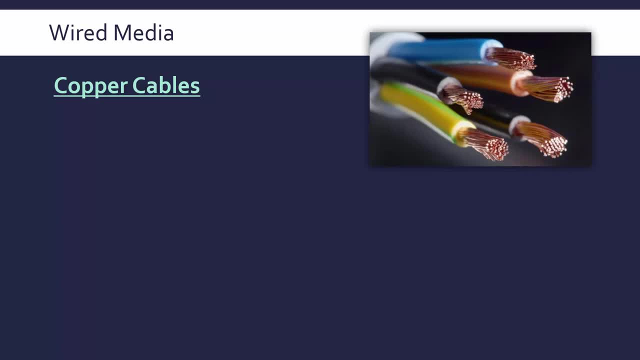 In this image we've got a bunch of copper strands and together they form a wire and then we've got a cable itself. So probably stating the obvious here. but data is transmitted through these cables using electrical signals, So the electricity is carrying our data through these cables. Ethernet will use copper cables for. 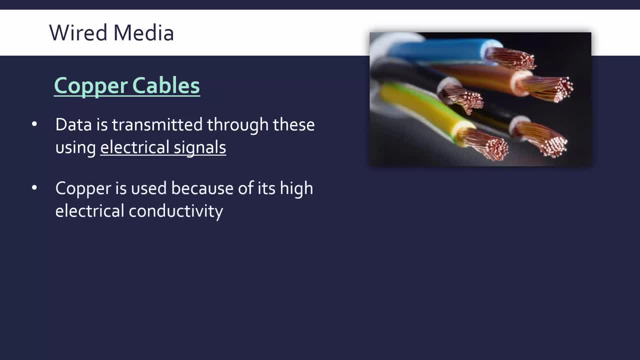 example, and copper itself is chosen as a material, as a metal, because it is good at conducting electricity. It has high electrical conductivity. It's not the most conductive substance. You could use silver, which is better. Gold is also good, but clearly they are more expensive and so it's a 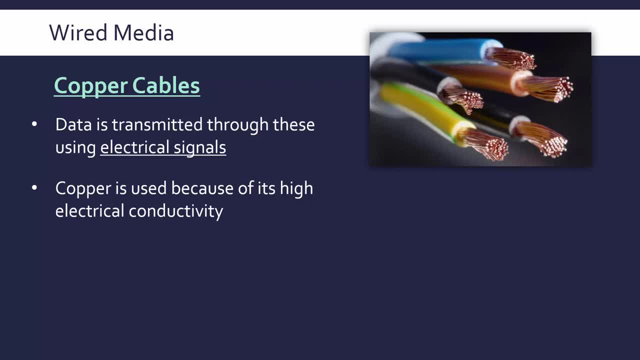 trade-off between a small increase in speed and performance versus a big increase in cost. One weakness to standard copper cables is because you've got all these strands, each of which is sending electricity. they can suffer what is called crosstalk, where one cable or one wire, I should say. 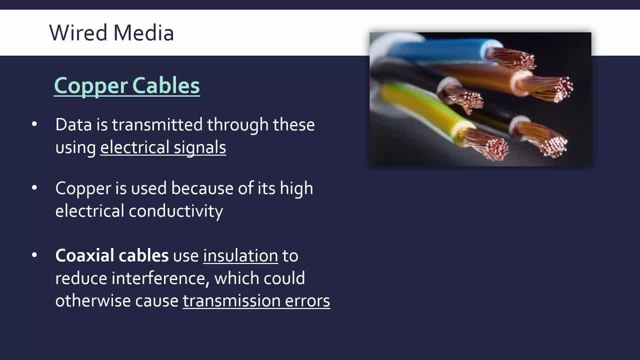 affects another wire and this interferes. So interference is a quite common problem where the data being sent degrades and suffers errors because it's being interfered with by signals which are spillover, you could say nearby. Now that will cause errors in your transmission if you send data and it 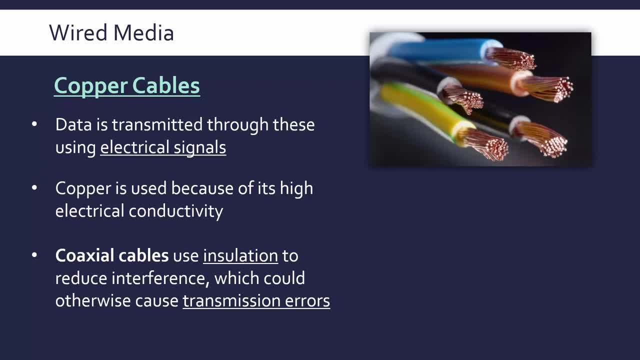 suffers interference. it won't arrive in the same way you are hoping it will, which can slow the network down. You've got to resend it, and that can take some time. Interference can happen with wireless connections too. Bluetooth and wi-fi can interfere quite a lot because those radio waves have got 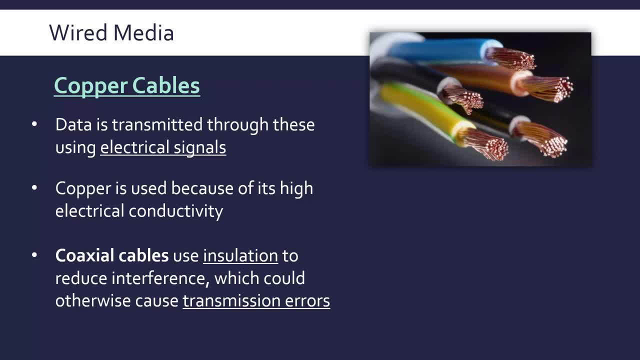 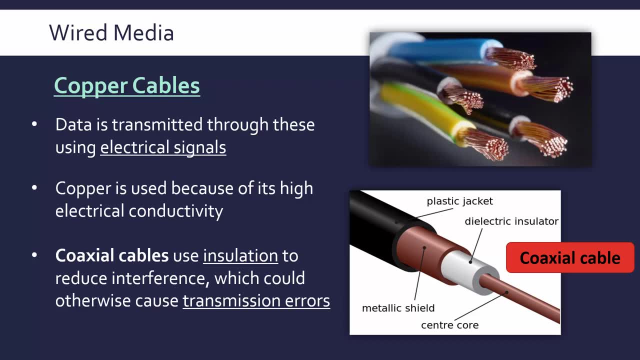 similar frequencies and can collide- at least you can picture it like that- which can also cause errors. So it's not just copper alone, but to mitigate it there is another, more specific type of copper cable called a coaxial cable, also called a coax, which effectively wraps a lot of insulation around the copper itself to try and prevent interference between separate 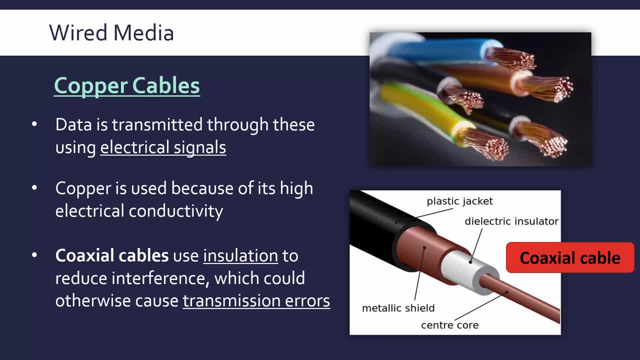 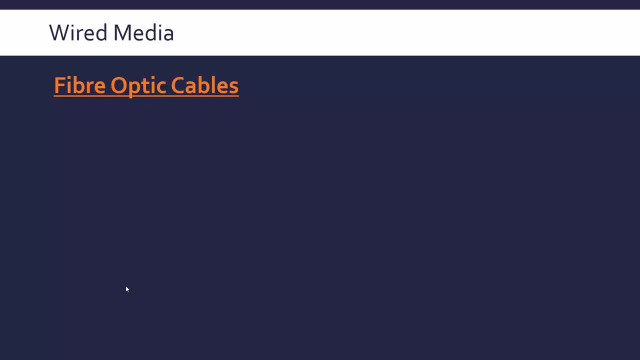 copper wires. This is a little bit more expensive, but can improve performance. Speaking of improved performance, the most high-end type of wired media are fibre optic cables. If you pay for better internet, you're probably paying for fibre optic. for example, It's often advertised, I'm sure. 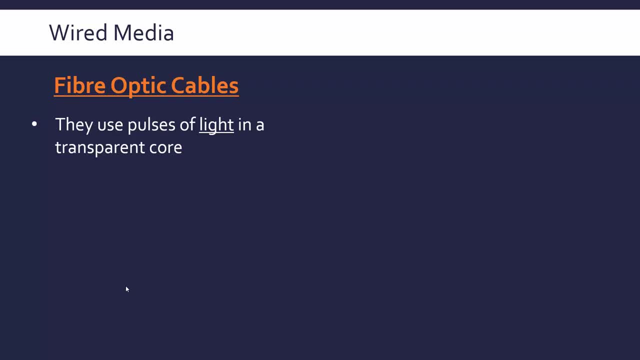 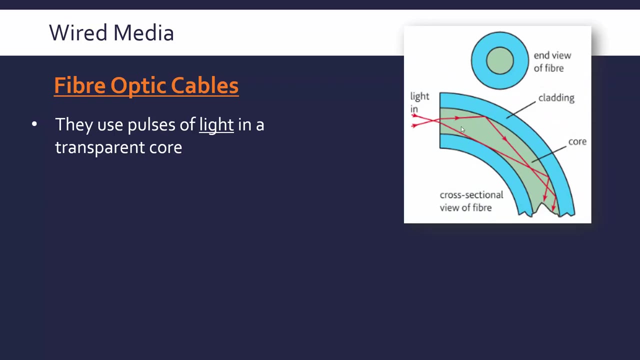 you would have come across that term before. So fibre optic cables, as the word optic would suggest, uses pulses of light to transmit the data instead of electricity. So no electricity going through these cables, it's just pulses of light and it's actually a transparent core which it travels. 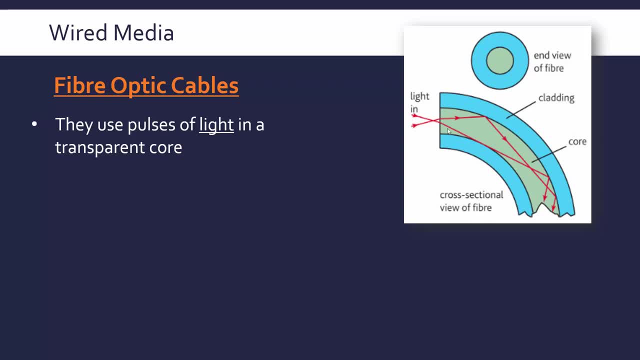 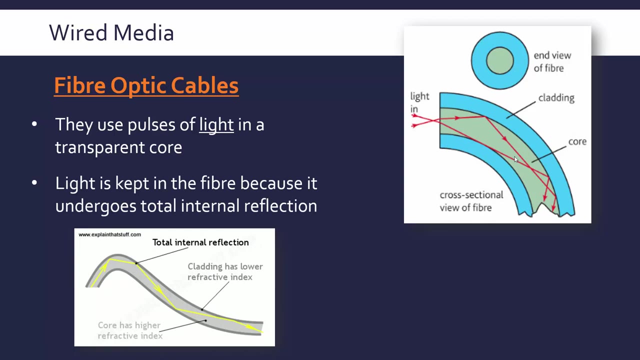 through and this core is usually some very light and flexible glass or plastic. in some cases It can be quite brittle, so it can break sometimes. Now, despite this core being transparent, just being glass or plastic which is clear, light is kept inside the fibre because the light is undergoing. 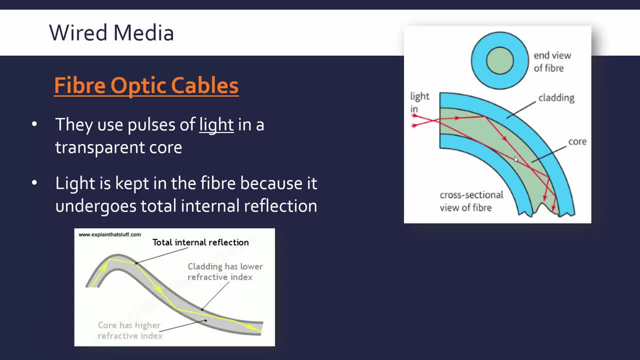 internal reflection in theory, total internal reflection where it's kept in because you've got the outside bit of the cladding with a lower refractive index. Now that's a physics topic so we're not going into that in too much detail, but it does mean these have generally got quite a good 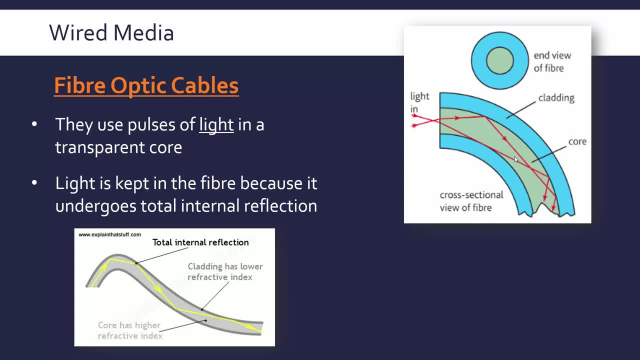 range because the light is not going through the fiber. but it does mean these have generally got quite a good range because the light is not escaping, although the range does degrade over time. because the material is not always perfect and it may not be total internal reflection, some of it might seep out.